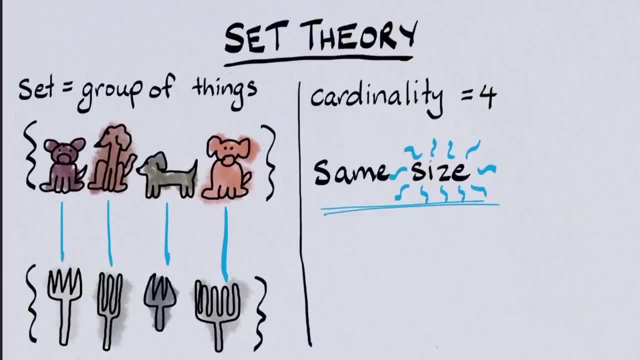 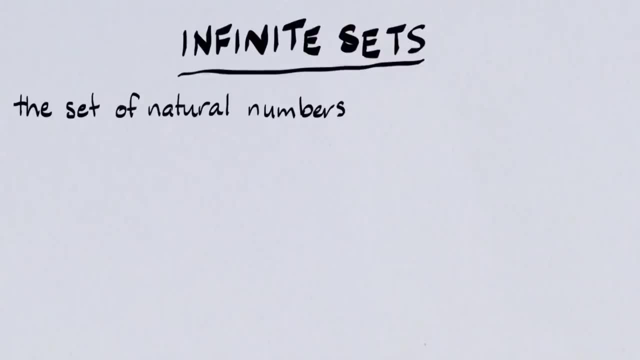 to be paired up with each other. You'll see why this is important right now. Let's look at a set with infinite cardinality, the set of natural numbers. It starts at one, or sometimes zero, depending on what textbook you're reading, and increases by one forever. 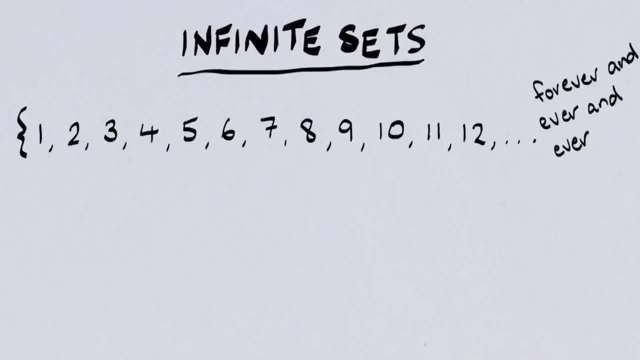 and ever and ever. This is totally allowed in set theory, by the way. we're not breaking any rules. Now let's look at another infinite set, the set of squares of the natural numbers. Every element in the second set, the set of squares, can be paired to a number in the 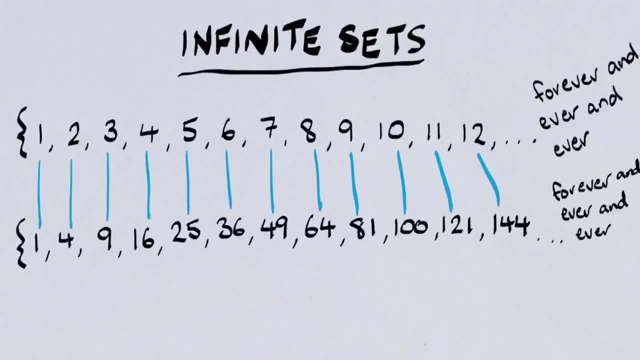 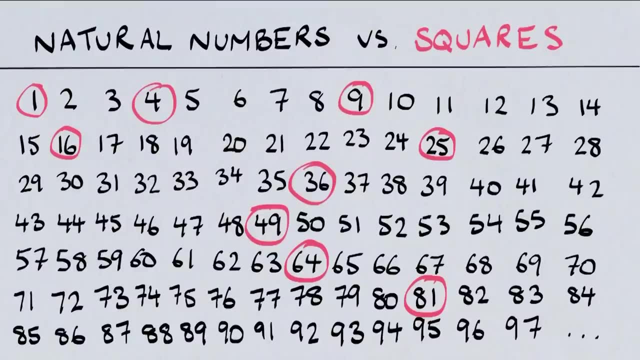 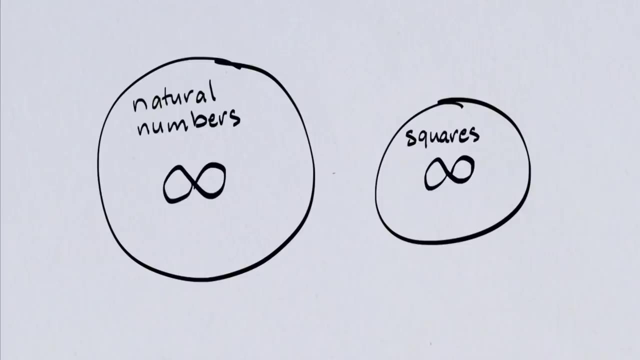 first set the set of natural numbers. So then according to our definition they're the same size, But intuitively this feels wrong. There are so many more numbers in the set of natural numbers than the set of squares. Is one set bigger than the other? But they're both infinite. 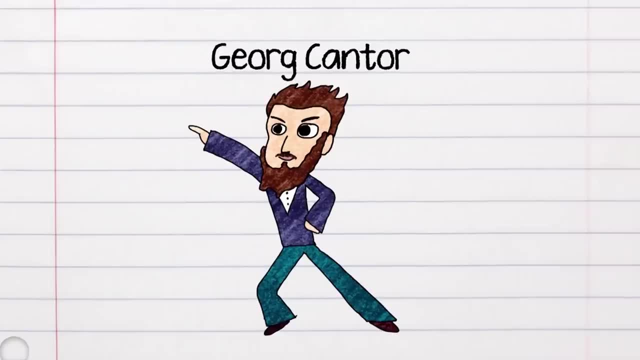 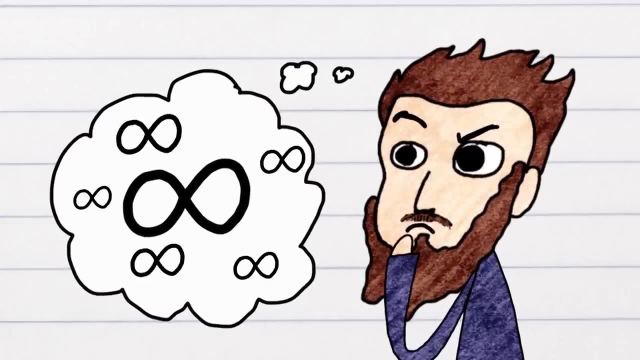 Infinity is infinity, right. It was at this point that George Cantor came along to save the day. He thought a lot about infinities, and actually legend has it that he thought about them so much that he drove himself insane, spending his last 20 years in and out of mental institutes. 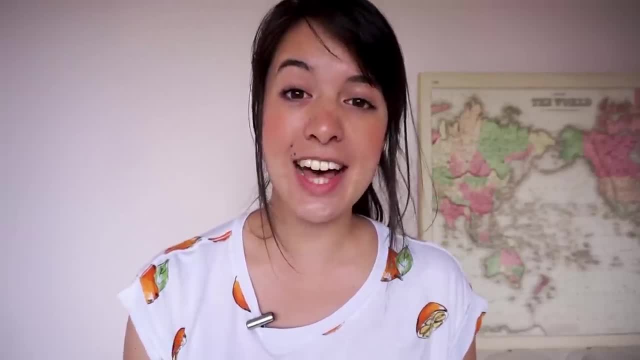 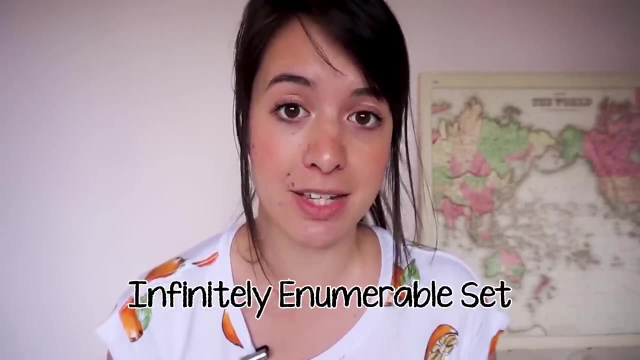 Remember him for his amazing work on numbers. He introduced the idea of an infinitely innumerable set. This just means a set whose elements can be paired off with the natural numbers. The word typically used is counted, because effectively that's what: pairing things off. 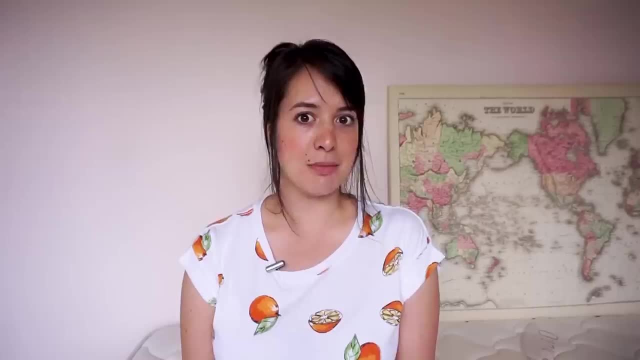 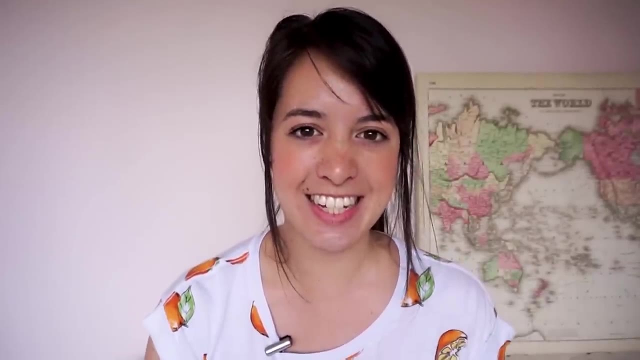 with the natural numbers is, But that's kind of confusing because you can't really count all the natural numbers. You die around 3 billion, So some prefer to call it listing, and I rather like this. Cantor declared that infinitely innumerable. 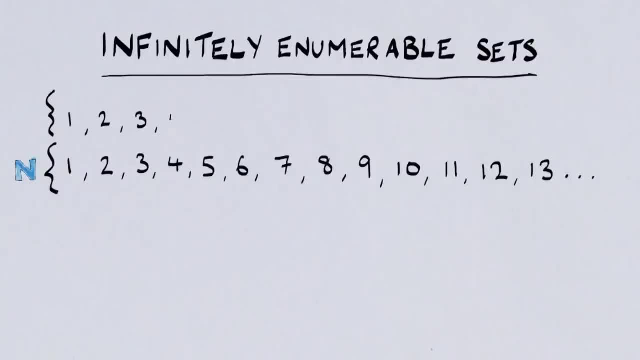 sets are all the same size. The set of natural numbers is obviously innumerable, as it can be paired off with the set of natural numbers. The set of squares is innumerable, as we showed before, so then it's the same size as the set of natural numbers. 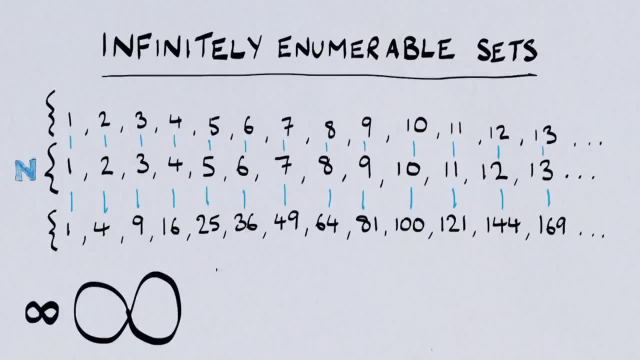 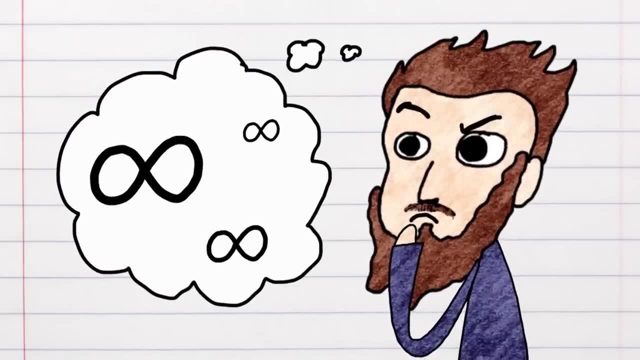 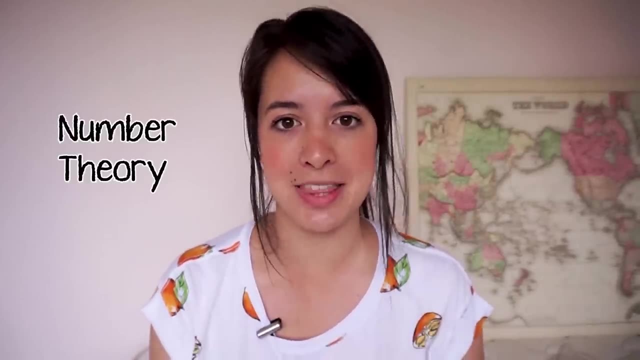 But are there some infinite sets that can't be listed? Are there different sizes of infinity? Cantor suspected there were. In particular, he wondered about the relationship between the set of natural numbers and the set of real numbers. We need to take a break from set theory to talk about number theory. 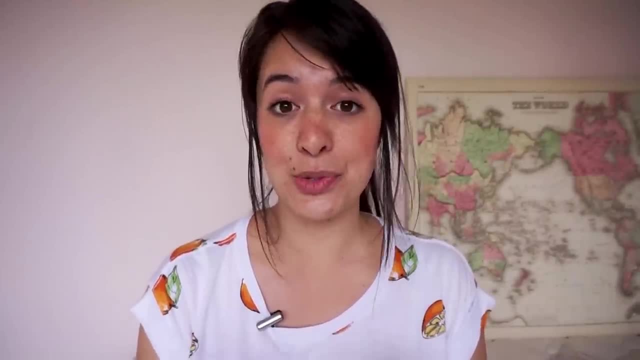 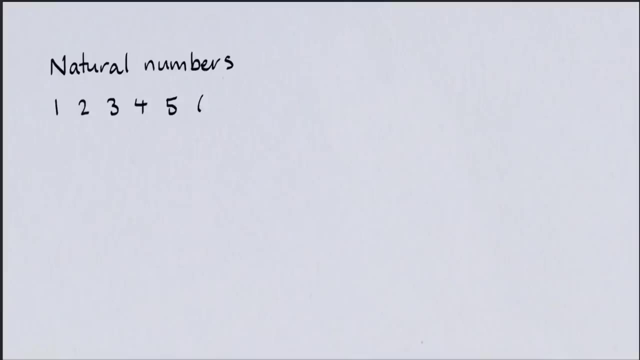 but don't worry, it's just as fascinating To understand Cantor's work. we first need to understand the different types of numbers and their relationship to each other. We've already talked about the natural numbers, whole numbers from 1 to infinity. Then there are the integers. These are the natural 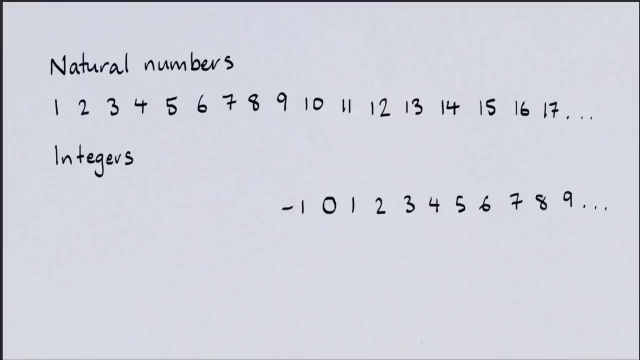 numbers. with the addition of the negatives, They increase all the way to infinity and decrease all the way to infinity. Then there are the rational numbers. These are just numbers that can be represented by a ratio of two integers. You might know them as fractions. All rational. 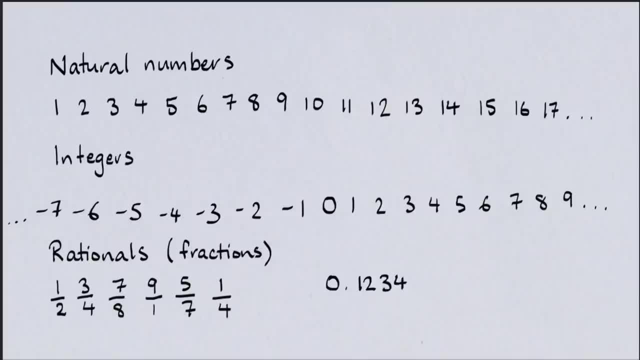 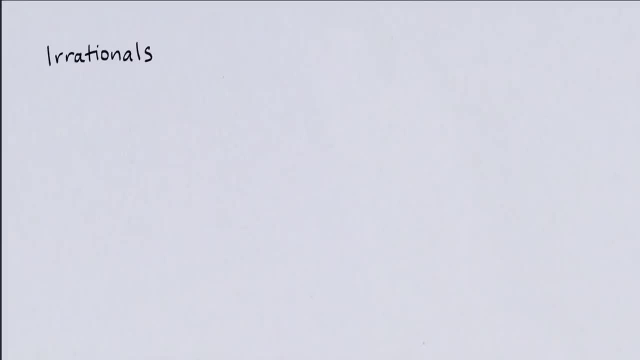 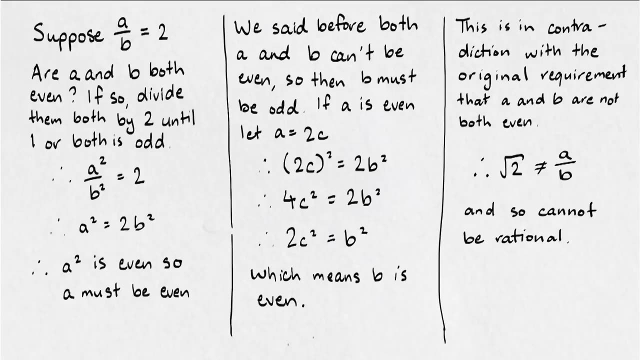 numbers can also be expressed as a decimal, with there either being a finite number of decimal places or a repeating pattern. Then there are the irrational numbers, which can't be expressed as a ratio of two numbers. Root 2 is a common example, and here's the proof of its irrationality. 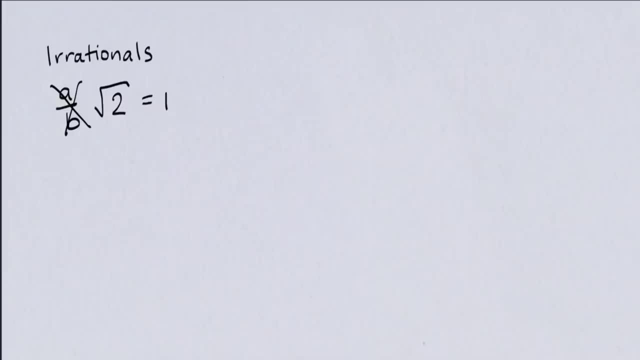 if you're interested. I think it's pretty clever If you express an irrational number as a decimal. the digits keep going on forever and ever with no apparent pattern. They're also sometimes called surds, which is actually from the word absurd, because the ancient Greeks really didn't. 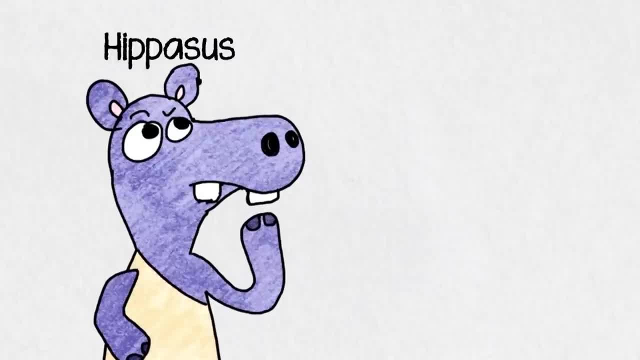 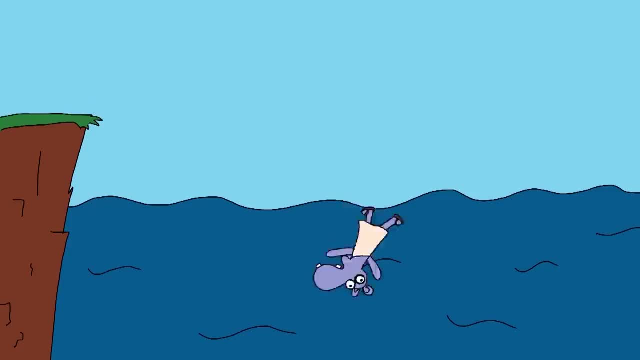 like them. According to legend, Pythagoras' disciple Hippapus was the one who figured out that root 2 is irrational and, to celebrate his finding, the ancient Greeks threw him into the Mediterranean Sea Like to drown. Yeah, they didn't like irrationals. 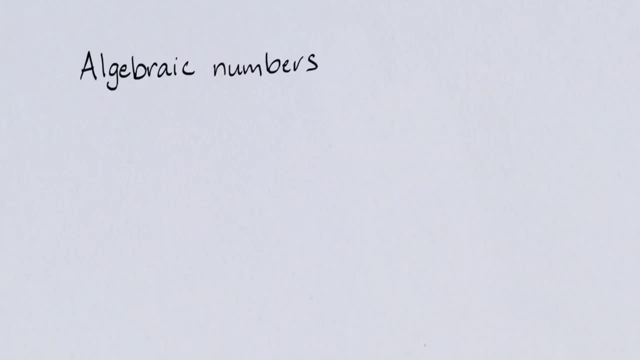 Then there are the algebraic numbers. These are just the numbers, which are solutions to algebraic equations. You know these things? They have one variable, usually x, and a series of terms that sum to zero, In this case 3.. Negative 3 is a solution to this equation. 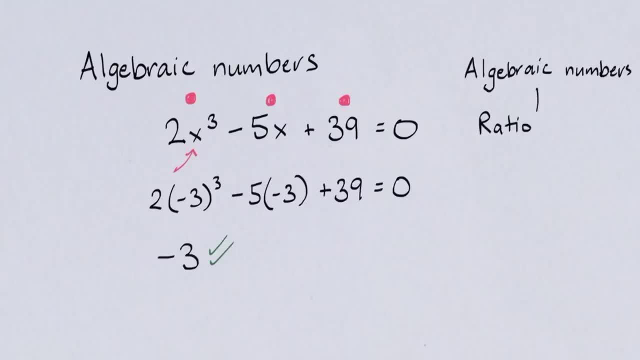 so it's an algebraic number. All integers and rational numbers are algebraic numbers. A lot of irrationals are too. So are there numbers that aren't solutions to any equation like this? Well, yes, there are In fact two of the most famous numbers: pi and Euler's number e. 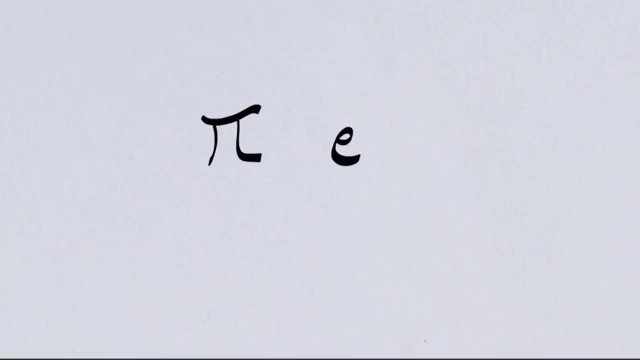 can't be calculated by any equation. These types of numbers have the coolest name of all: transcendental numbers, called so because they transcend the algebraic. All of the numbers I've talked about make up the real numbers. Here's a diagram to clarify things. 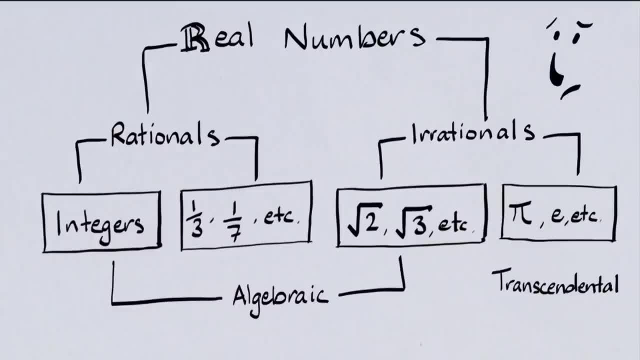 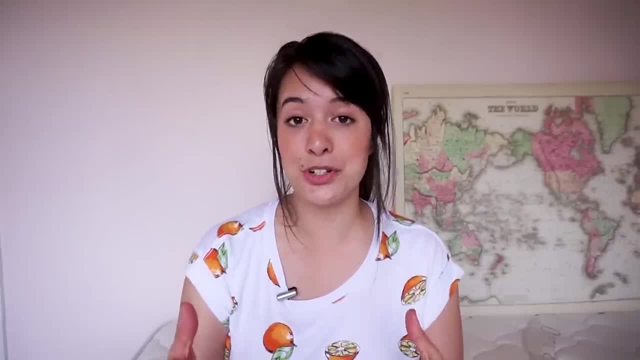 There are also the imaginary numbers, but they're not important here. Okay, then, now that we know about the reals and all of the numbers they're made of, we can get back to infinity. Now, Cantor wanted to know whether the set of real numbers was. 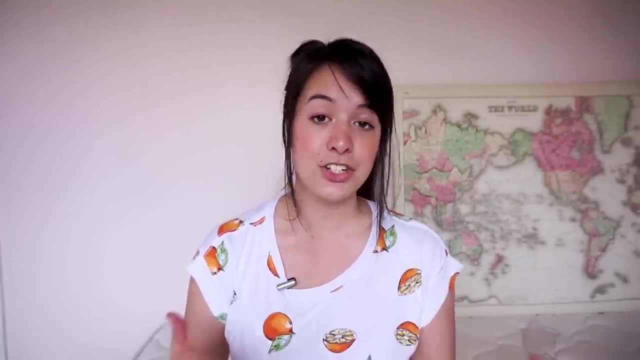 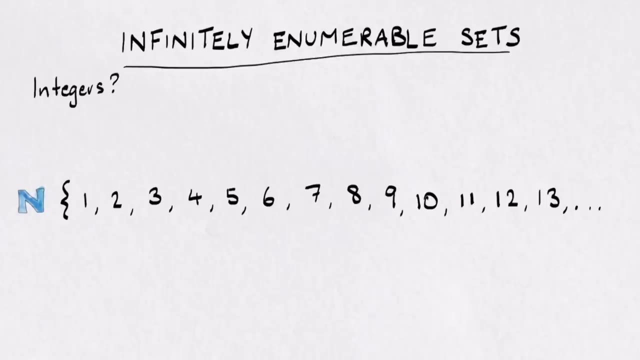 equal to the set of natural numbers, just like the set of squares. Well, let's take small steps, shall we? But like, not in a patronising way. Can the set of integers be paired off with the natural numbers? This isn't the usual way one. 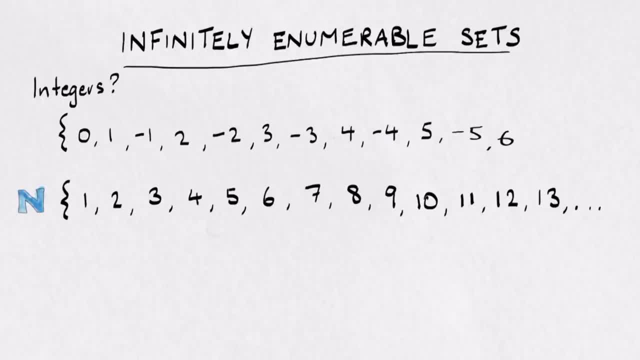 would write out the integers, but if we keep going with this pattern, we'll eventually write them all out. So yes, the set of integers is infinitely enumerable. How about the set of rational numbers? Surprisingly, they too are enumerable, If 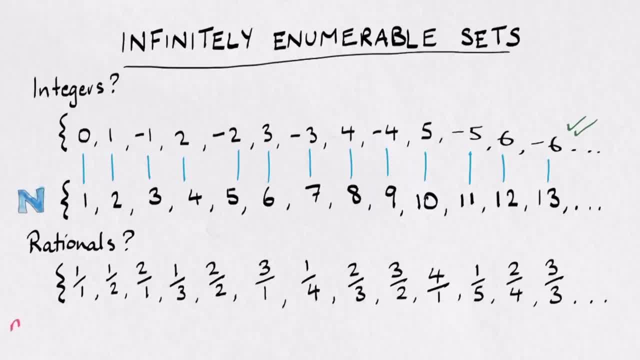 we write them out in this rather unconventional way, we can see that with the first element, the numerator and denominator add up to two. The next two elements have numerators and denominators that add up to three. The next three elements' numerators and denominators- add up to. 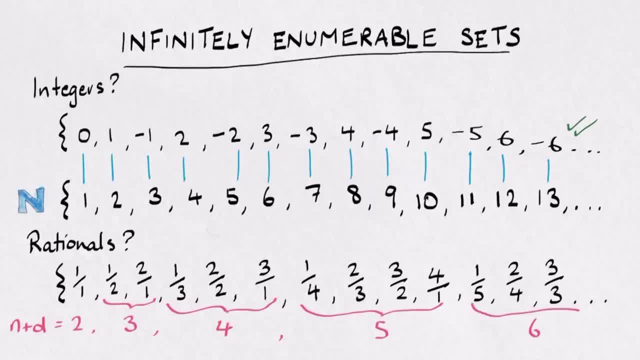 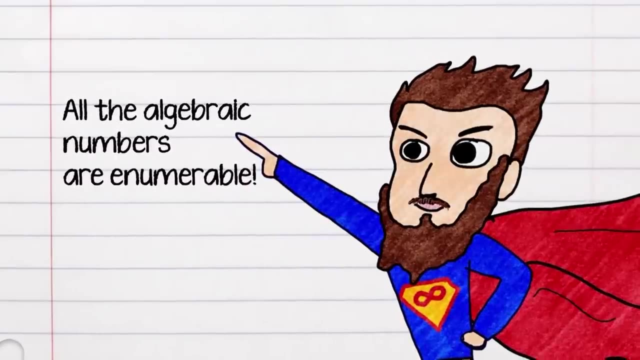 four. A list that continues like. this contains all the positive rational numbers. We can just include the negative rational numbers too, if we alternate, like we did with the integers. So then the set of rational numbers are enumerable too. Cantor even proved that all the algebraic numbers are enumerable. 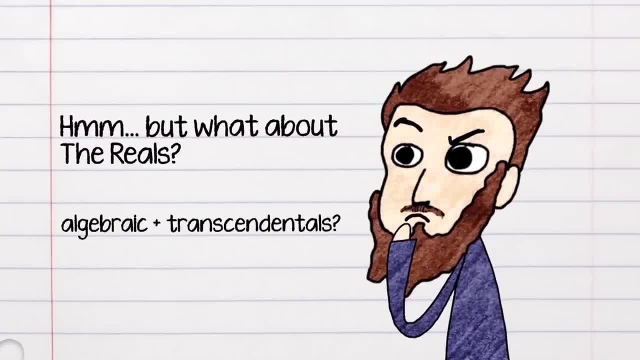 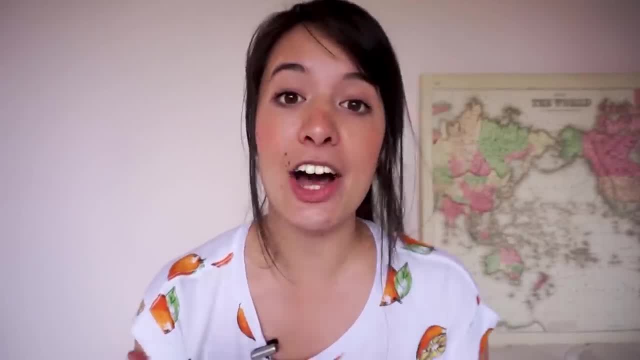 So then, what about the reals, which encapsulate both the algebraic and the transcendental? In the same paper, he proved that the real numbers are not enumerable. They are in fact a different kind of infinity, imaginatively called non-enumerable. 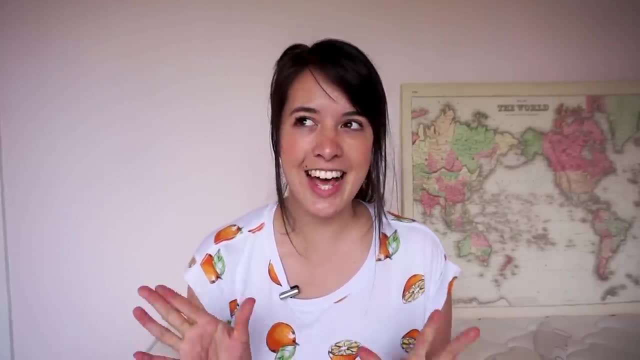 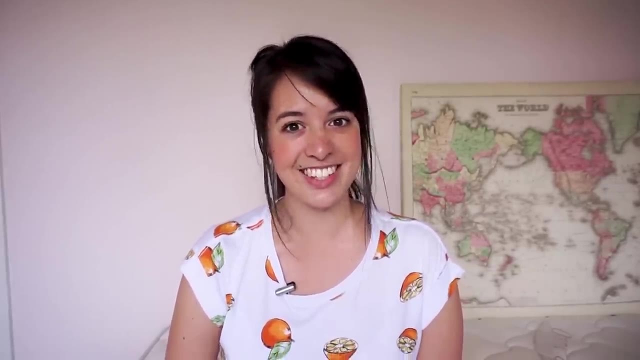 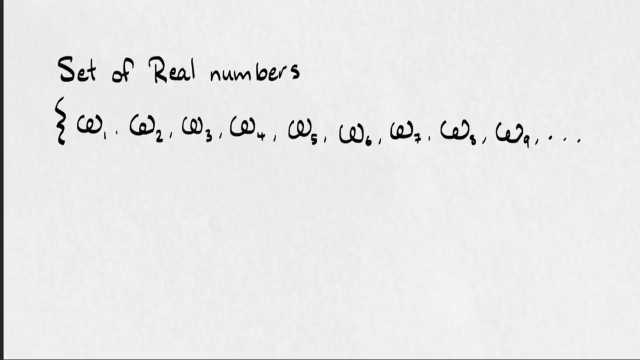 Cantor was a huge fan of proof by contradiction and he had an inkling that the reals were non-enumerable. So of course he started the proof with the assumption that the reals are non-enumerable. So if we assume that the reals are non-enumerable, we can pair them off with each of the natural. 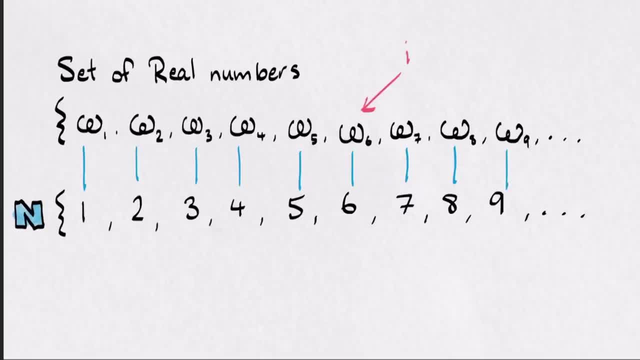 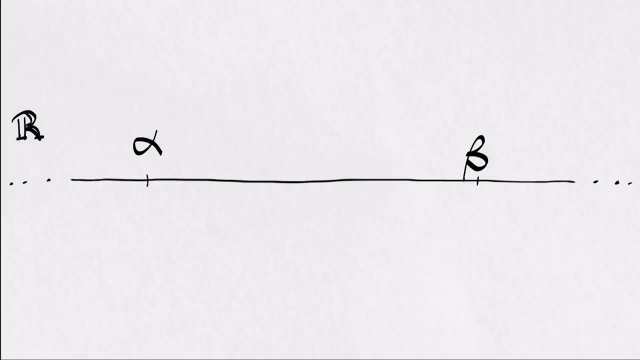 numbers. Cantor showed that this list will always be incomplete. Pick any number alpha and any larger number beta and mark them out on the real number line. This is just the list of real numbers marked out on a line. Now find the first real number on your list that is bigger than alpha and the first real number that 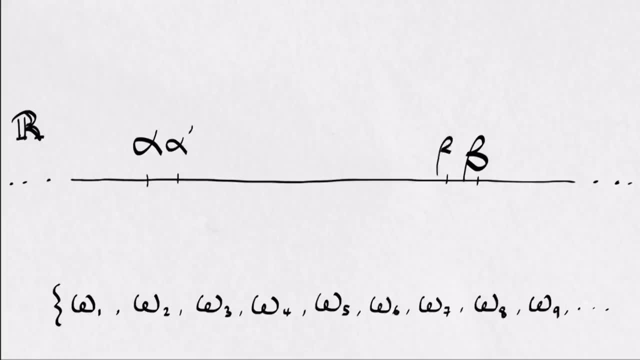 is smaller than beta. We'll call them alpha prime and beta prime. Do this a couple more times. Now the thing is, you'll always be able to find two more numbers between the last two numbers. Suppose you get stuck where v indicates around a trillion prime marks, but a finite number. 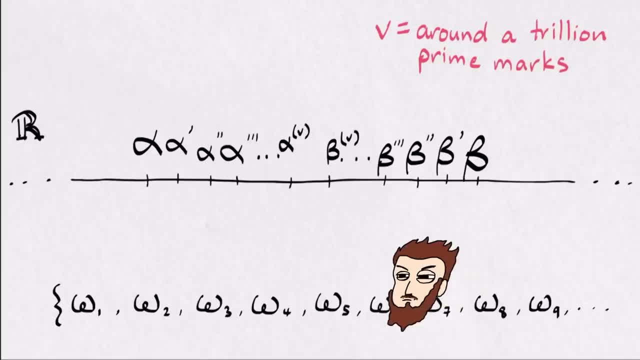 Now, no matter how hard you search through the list of enumerated real numbers, you can't find another one larger than alpha v and smaller than beta v. So then are there no more reals between them? Well, what about alpha v plus beta v on 2, the average? Your list is missing that number. 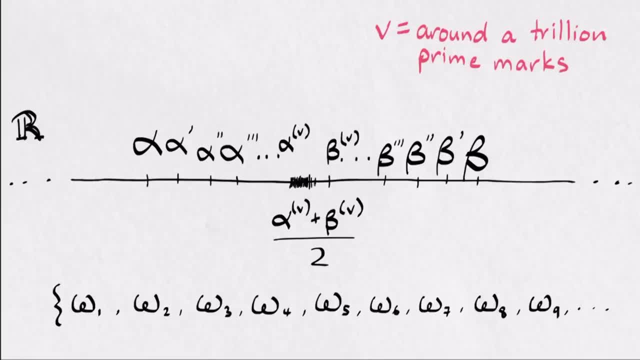 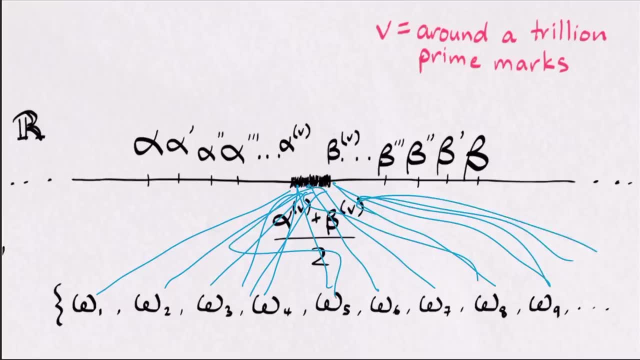 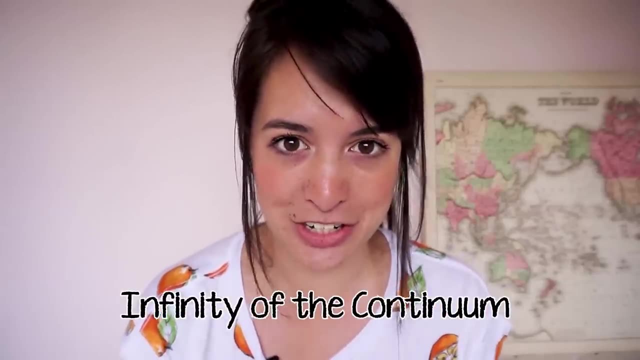 And then what about all the numbers between alpha v and the average and beta v and the average? This could go on forever. It doesn't ever stop. There are an infinity of numbers between alpha and beta, and between alpha v and beta v. This is called the infinity of the continuum, and we can't pair. 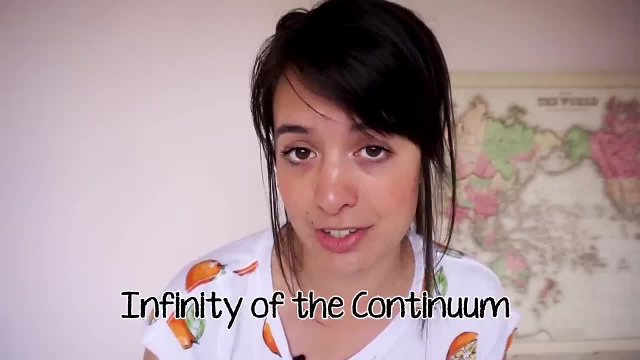 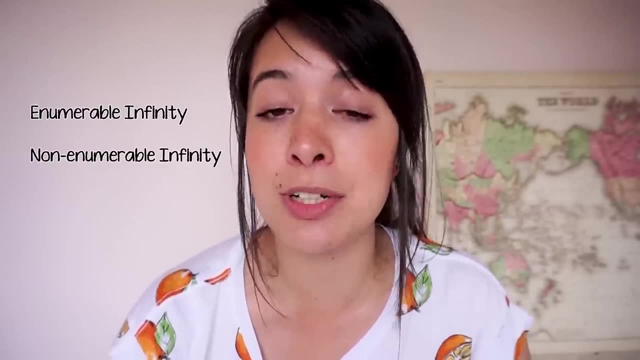 it off with the natural numbers the way we could with the integers and the rationals. There are a two types of infinities: the enumerable infinity of the natural numbers and the non-enumerable infinity of the continuum. I really like this proof because I think it conveys the intuition. 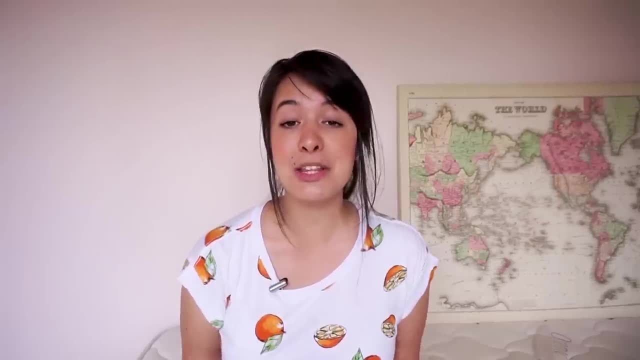 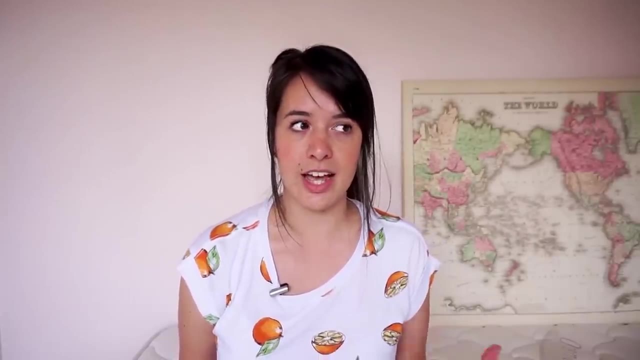 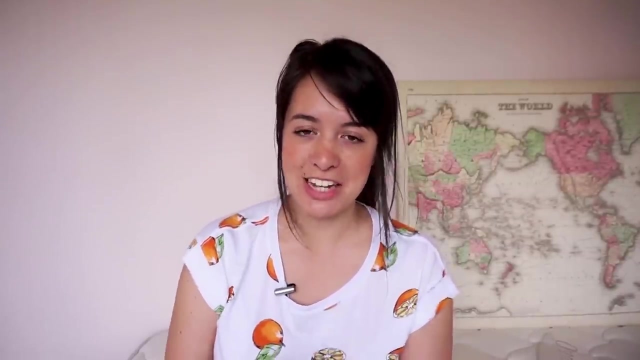 really well, but it is also pretty abstract. so there's another proof I want to show you too. You know, just for fun. It's called proof by diagonalization, or the diagonalization proof, or diagonalizing. It involves diagonals. Canto again begins by assuming that you're going to be. 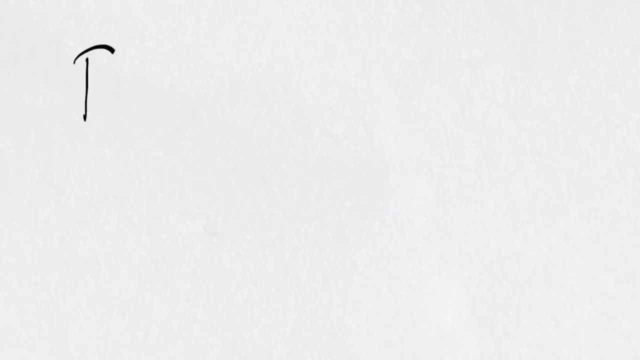 able to number all the real numbers on a list. In fact, he restricts it to just real numbers between 0 and 1.. We can't really do this in order, because the first number would be a point, followed by an infinite amount of zeros with a 1 at the end, which would take an infinite amount of paper. 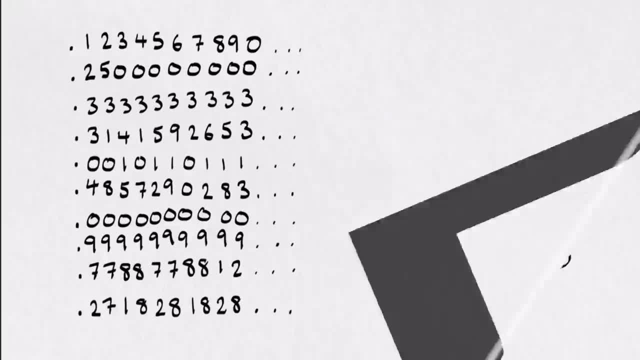 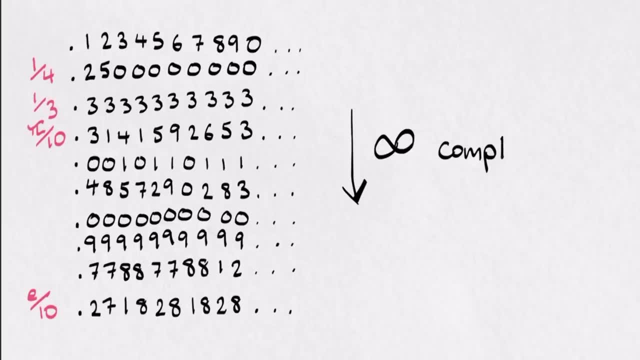 and ink to write. So let's just choose randomly. These numbers are pretty good. It's got a quarter, a third, pi on 10,, e on 10.. It's infinite. But is it complete? Nope, And this is how Cantor proved. 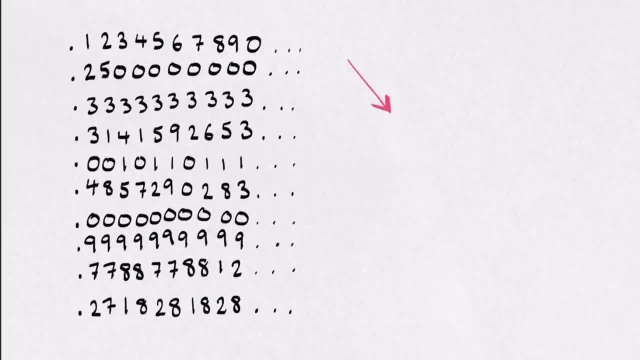 it. He went down the list in a diagonal fashion, selecting the appropriate digit, For example the first digit of the first number, the second digit of the second number, the third digit of the third number, and so on, And then he used them to create a new number. Then he added one. 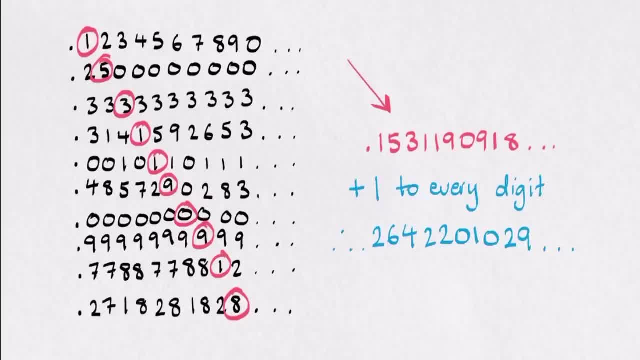 to every digit. Now is this new number on the original list. Well, let's do a rigorous check. Is it the first number? No, because the first digit of the first number is 1, and the first digit of the second number is 2.. All right then. is it the second? 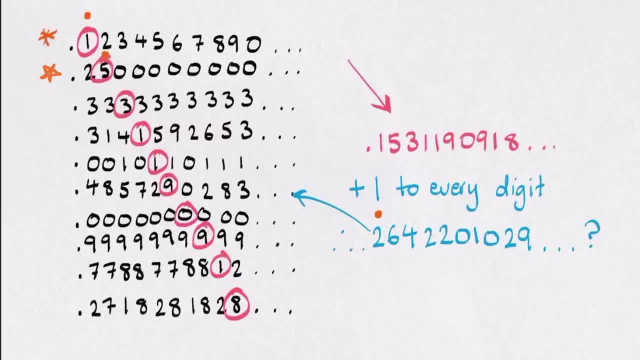 number? Well, no, because the second digit of the second number is 5, and the second digit of the new number is 6.. It's not any of the numbers. We've found a number that isn't on the original list. 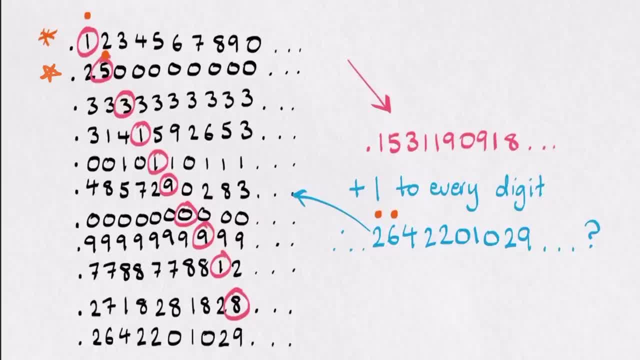 so let's add it on. Now is the list complete? Well, you can just repeat the process and find another number that wasn't on the list. By coming up with new digits in this diagonal fashion, you can always find another number that isn't on the original list. Therefore, our list can never. 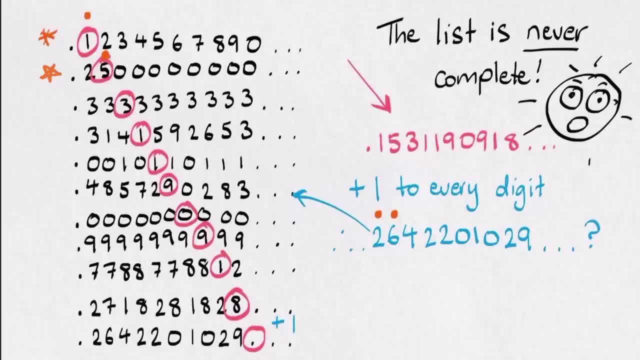 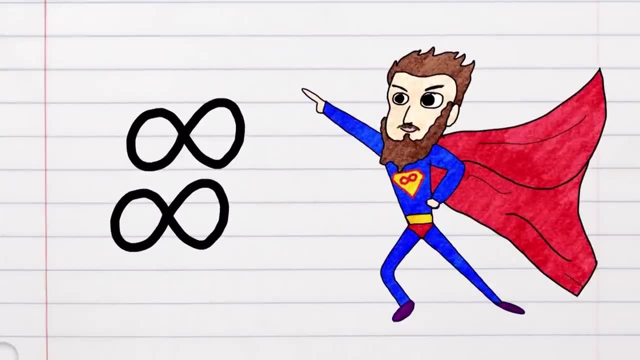 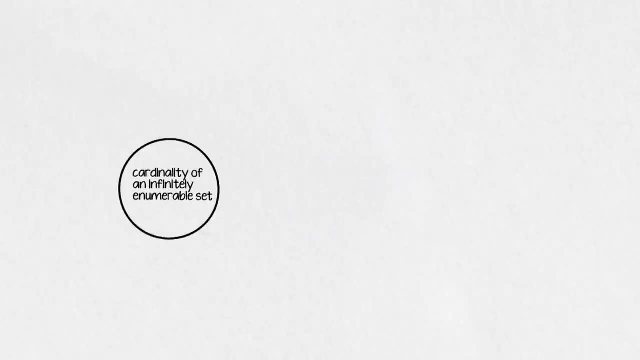 be complete, There are always numbers that aren't in it. It's impossible to list all the real numbers between 0 and 1, let alone 0 and infinity. Cantor also showed that not only are infinities different, some are infinitely bigger than others: The cardinality of an infinitely innumerable set. 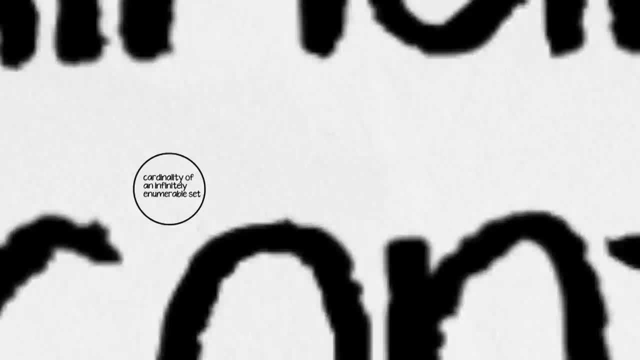 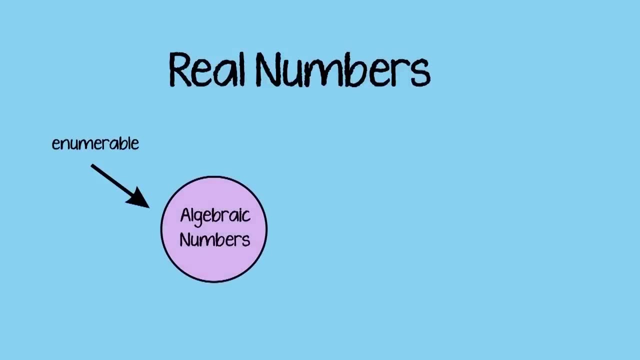 is smaller than the cardinality of the continuum, but like a lot smaller. Yet the only difference between the algebraic numbers, which are innumerable, and the reals, which aren't, are the transcendental numbers. So what does that mean? 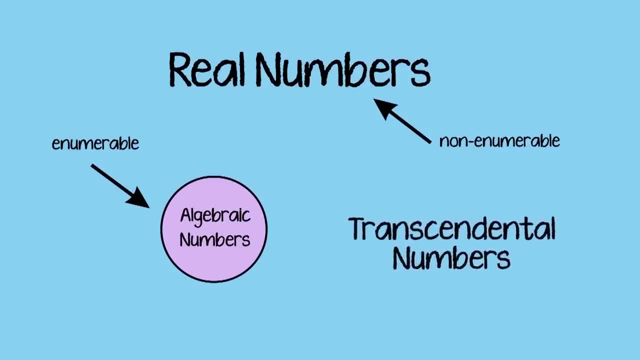 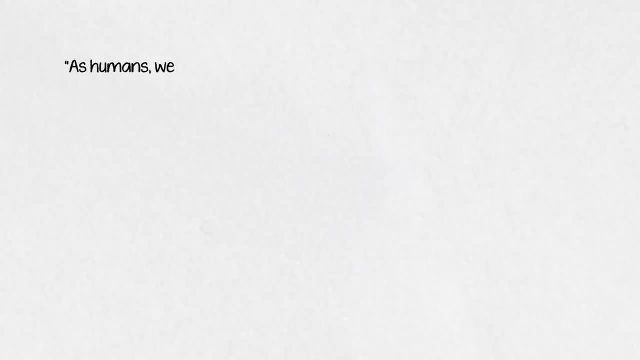 It means that transcendental numbers make up pretty much all possible numbers. Now I want to wrap up with a quote from the book I got most of my information from. As humans, we value neatness, order and patterns. We're interested only in numbers. 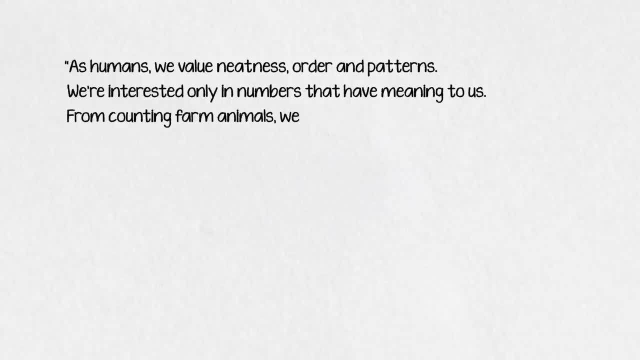 that have meaning to us. From counting farm animals, we have invented the natural numbers. From measurement, we have invented the rational numbers. and from higher mathematics we have invented the algebraic numbers. We have plucked all these numbers from the continuum, while ignoring the vast depths. 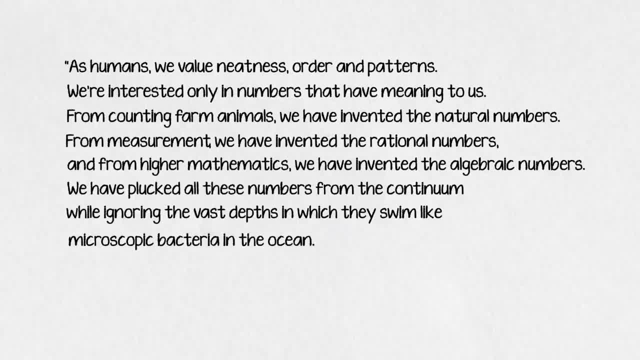 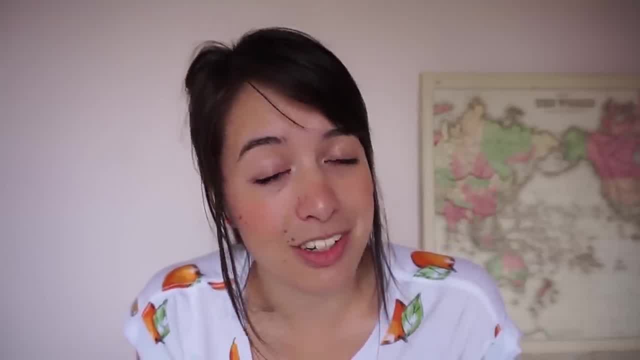 in which they swim like microscopic bacteria in the ocean. Virtually every number is transcendental. I don't know. I think that's pretty cool. I must say this was probably my favourite video to make because I found the topic so fascinating.